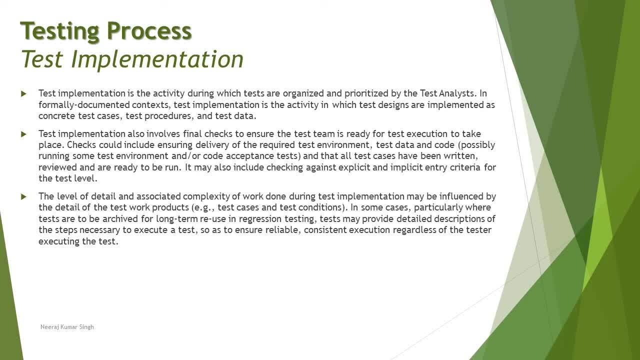 then, what kind of teams do you have, what kind of availability of the team you have, whether everyone is ready to get going for the execution or not. Even you check on the availability- availability of the test environment which you will be using in order to run, Because, of course, 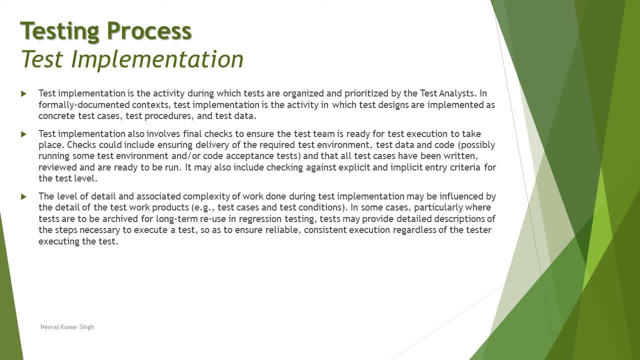 you might have different environments at different point of time to conduct different levels of testing. So you do make sure that at least with the initial level of testing, like unit and integration and so on, you have the environment set up and ready to use, and definitely that becomes. 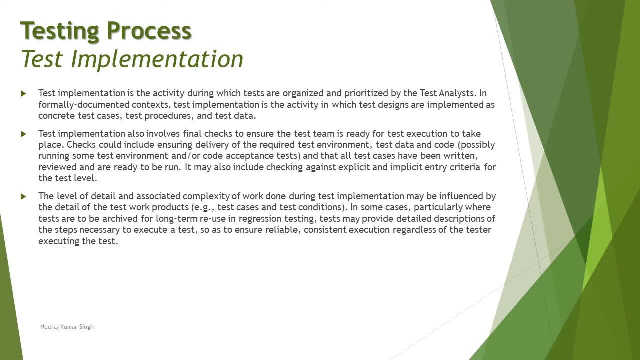 a very important factor in case of like entry criteria, to determine to start with a kickoff with the test. Moreover, even the level of details and the associated complexity of each work item will determine how exactly your execution will go on, Because if you have a lot of detail involved of 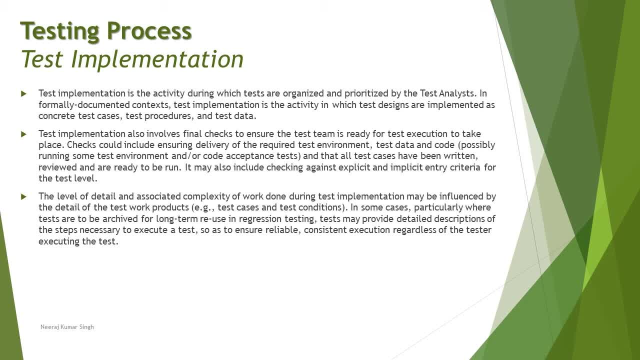 course, it is going to consume a lot of time to execute, and more importance given to those test cases which probably have more detailed infrastructure and information involved, Because a tester has to be very careful with all these details in order to create a scenario when executing these test cases. 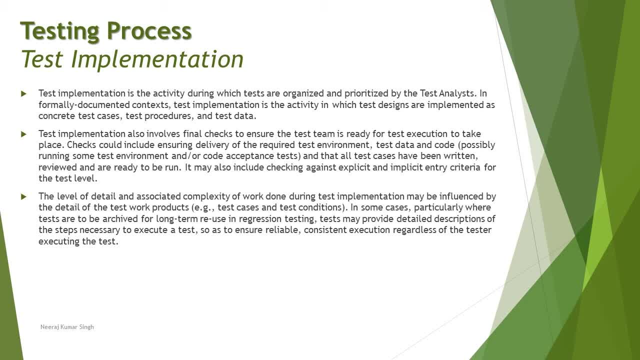 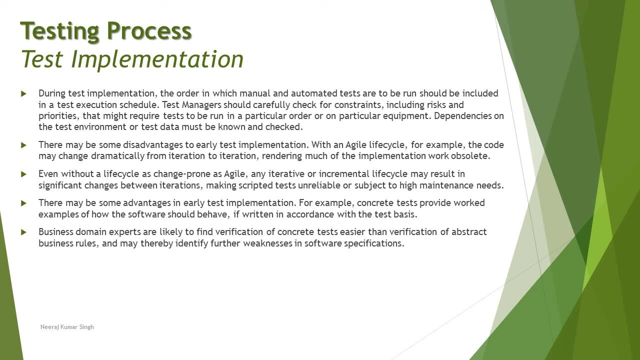 So these all factors, depending on the level of detail provided to you, will also influence the execution and, in fact, definitely let you know, log the same kind of details in order to satisfy the conditions. Plus, of course, we do have the ordering and the sequencing of the test cases. 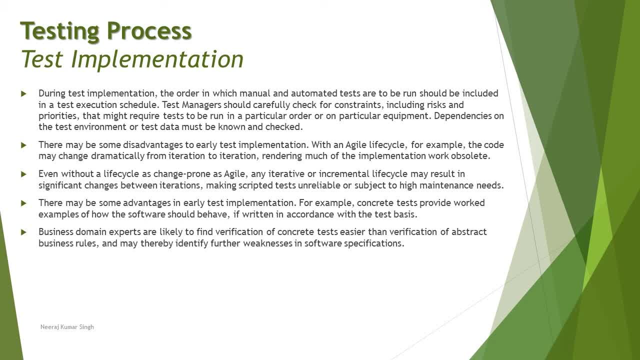 which you created in the previous stage, and this prioritizations and sequencing of the test cases is generally documented in a form of test cases Test Execution Schedule. Now, Test Execution Schedule not only deals with prioritization based on the risk or any other complexity factor. You do have a lot of other things which involves here is like: 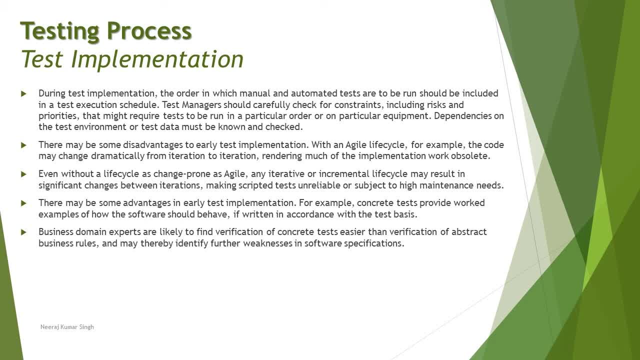 the dependency. Now again, dependency deals with technical dependency, logical dependency, and that would definitely help and add more value to this. Now, at this point of time, a test manager should be very careful to check any of the constraints which might be involved in order to determine the performance of the test. 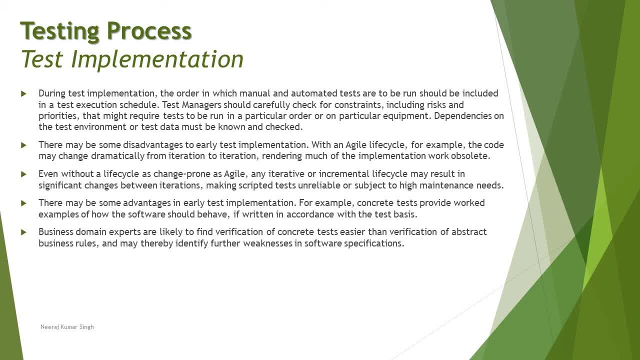 Prioritization, Because not just everything comes with the flow. Lot of things has to be considered and taken care of with the test manager in order to make sure that all the factors which influences your execution order or sequencing of a particular test cases, then definitely that constraints. 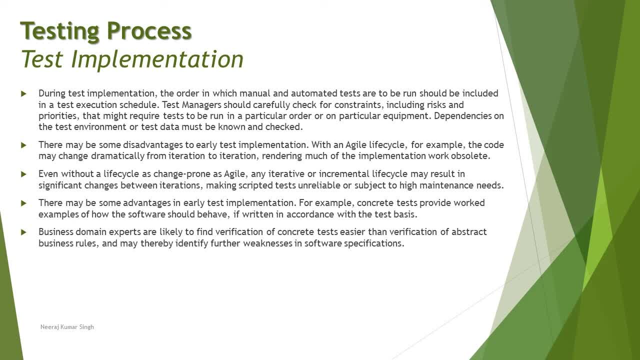 must be considered before creation of the test schedule And even if it is created. if you see, as for the i-stqb, they say that the testers are the ones who create test execution schedule. the test manager can definitely have a quick check on these things which are being created. 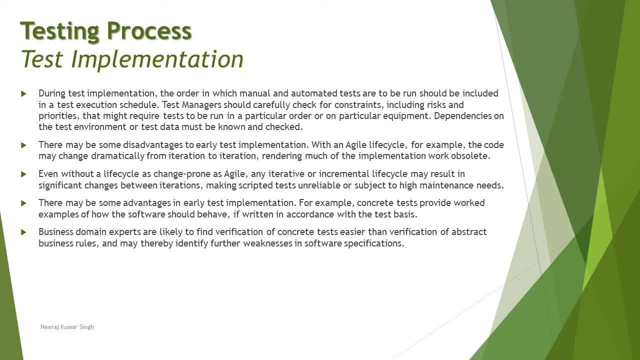 to finally determine the right order and making sure that everything is well established in order to run the test smoothly. there are many other disadvantages of early test implementation as well, so in the previous cases, previous stage, we understood that test implementation can actually begin before the end of test design. but what could be the disadvantage of having early test? 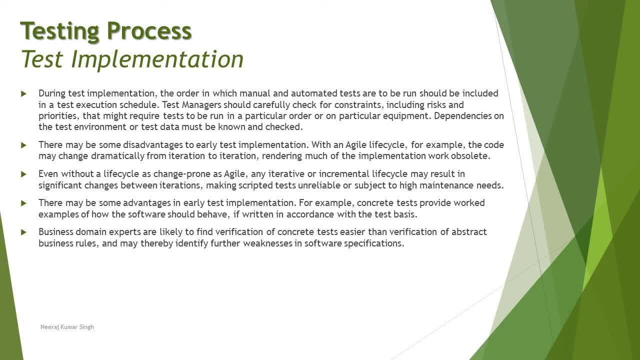 implementation happening. so with an agile life cycle, for example, the code may change dramatically for from iteration to iteration, rendering much of the implementation work absolute. now, of course, you know, when you have frequent changes involved in your project, early implementation could sound bane and rather you need to rework a lot of things at any point of time to fulfill the need and 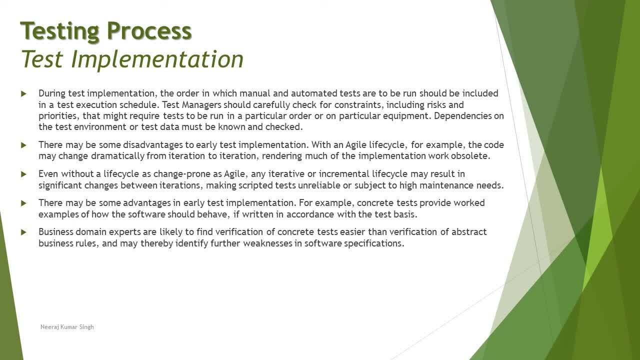 expectation of the requirement or probably the code, because even if you run those test cases might not be applicable with the new code which has evolved between the iterations. so that's one of the thing, and even without a life cycle which is, uh, as change, prone as a job and any iterative or incremental life, 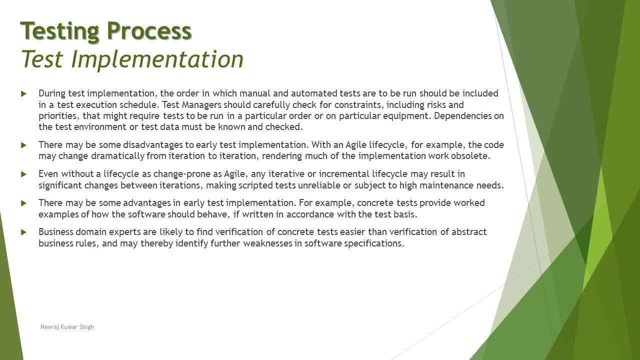 cycle may result in significant changes without iterations as well, or between iterations, making scripted test unreliable or subjected to high maintenance needs. so these are all the factors which could be considered as one of the demerits of starting implementation early, but, at the same time, it's a great way to start implementing early, but at the same time, it's a great way to 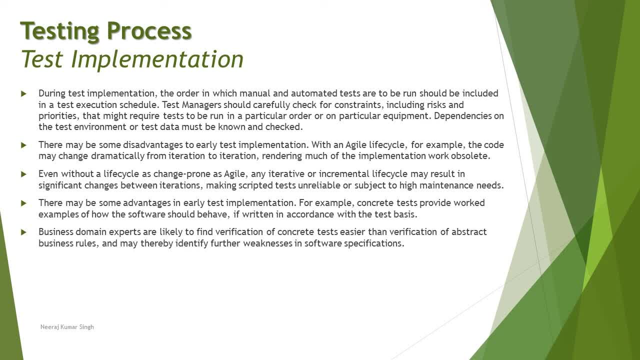 time, you cannot ignore the advantages of having early implementation. for example, concrete test cases provide worked examples of how the software should behave if written in accordance with the test basis. it could be really helpful, and business domain experts are likely to find verification of concrete test cases easier than verification of abstract business rules. so you know, of course.